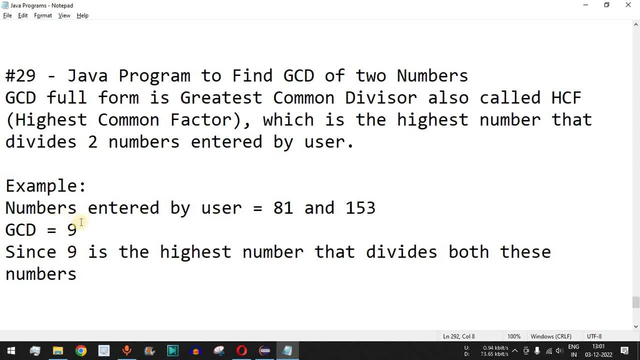 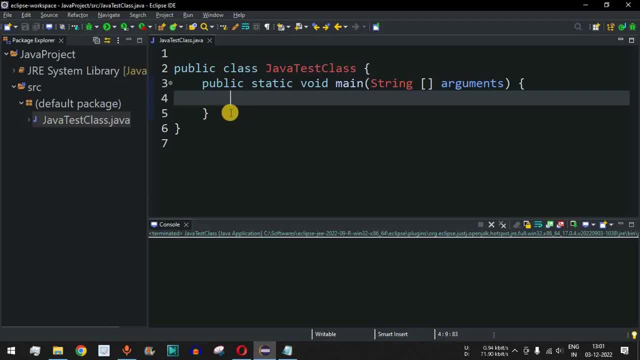 highest number that will divide both these numbers. So, ultimately, we will be finding that 9 will be the number which will be dividing both these numbers over here. So, guys, let us move to the eclipse id in order to implement this algorithm over here. So, first of all, we will declare two: 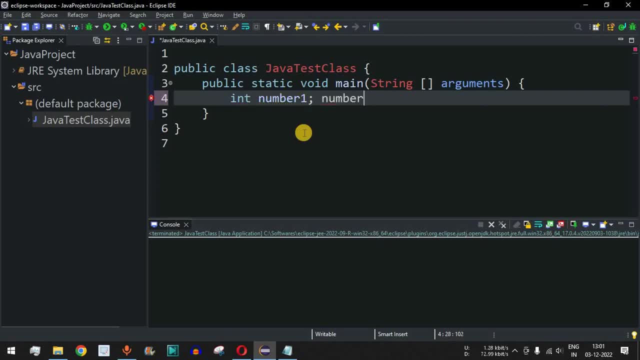 numbers over here. So we will say number 1, and then we have number 2, in this case, and then over here, instead of semicolon, we will be having our comma over here and then we have semicolon at the end of the line of code over here. Now we will ask the user in order to provide the first number. 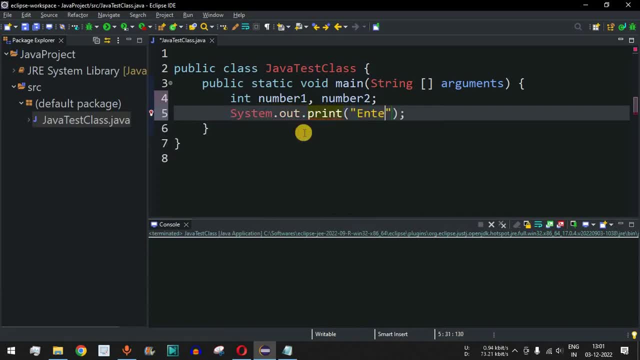 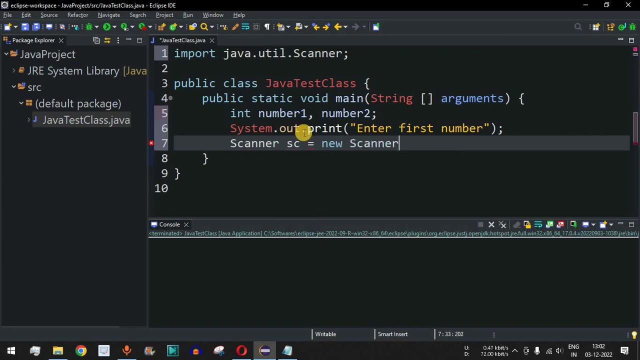 so we will say enter first number over here as the label. So we say enter first number and then followed by: we will be using our scanner class in order to take the input from the user. So scanner will be the class equal to new scanner in this case, and then we will be having systemin so that 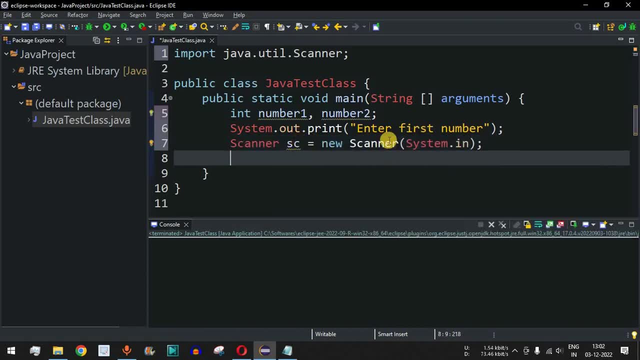 the user is able to provide the input on the console. So first the user will be asked to provide the first number over here, So we will be using our number over here, and then we will be asking the number 1 as the variable equal to, followed by scnextend. So, guys, this is the line. 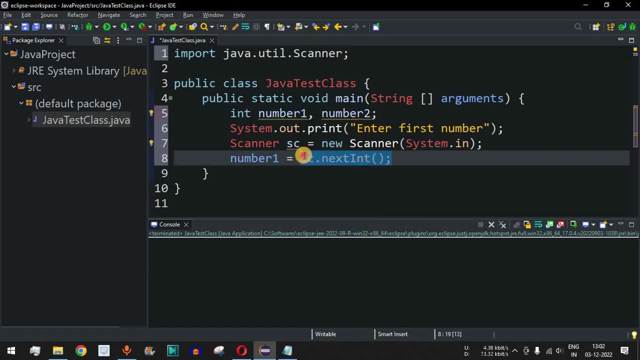 of code that is responsible in order to take the input from the user and it will be assigned to this number 1 variable. Now the next number. we will be asking the user once again to enter the second number over here, So we will simply copy and paste this line of code: enter second number. 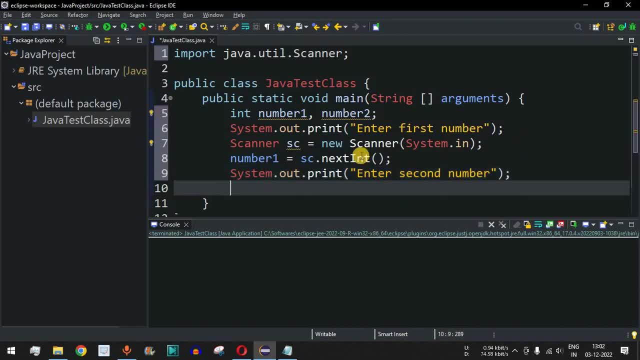 in this case. So it will be enter second number and then again we will be copying this line of code. So we will check whether it is this line of code or not by click on enter. Either of the ंas- the first one or this middle line, will be assigned to number 2 in this case. So we will be. 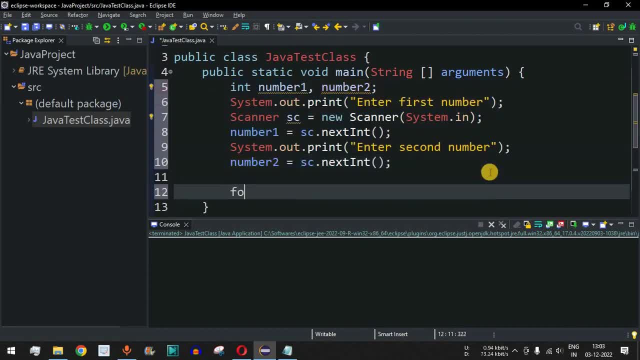 changing the variable, that is, to number 2.. So, guys, using these lines of code, we have got the two numbers from the user. Now we simply have to find the gcd. so how do we find the gcd? we will simply start with the for loop and int I- it is equal to 0- and then we need to check whether 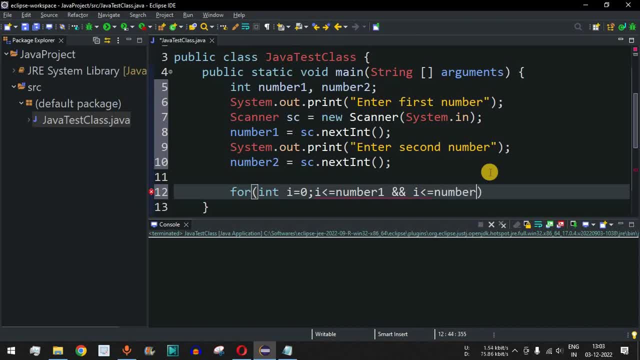 this i was, or equal to number 2. so, guys, this condition is very important. that's because we need to find a number that is less than both these numbers, but it is the highest number, which is dividing both these numbers over here. so this is: 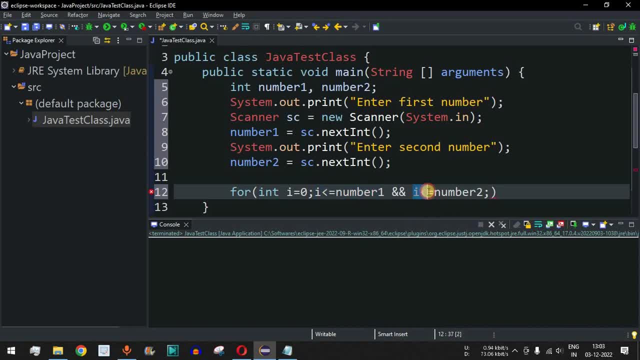 the condition that is, I is less than or equal to number 1, and it can also be I less than or equal to number 2, so both these conditions should be satisfied, and then we will be saying I plus plus. now. inside this for loop, our logic will be: 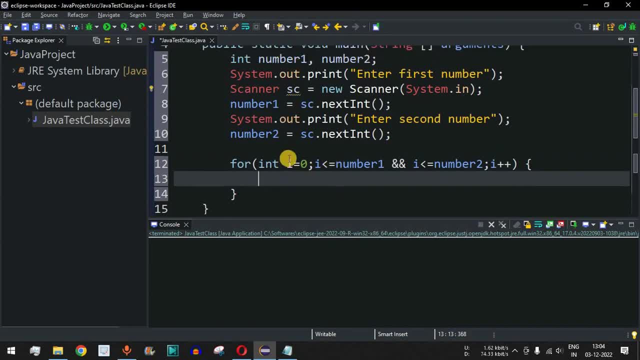 we have to check whether both these numbers can be divided by this number. that is I over here. so what we will do is, before this for loop, we will say int, GCD in order to store the GCD of both these numbers over here. so we will be. 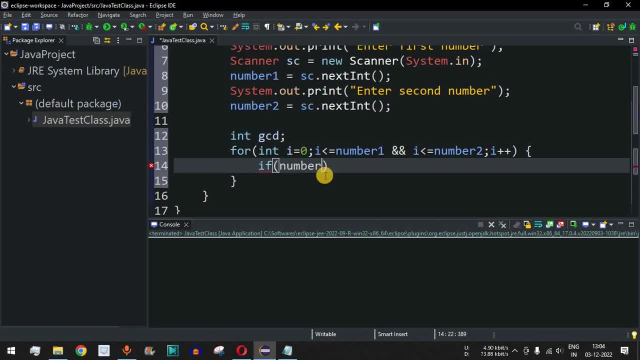 having our if condition over here. if, first of all, number 1 percent I is it equal to 0? this condition, and again, this number, that is same number, this number, that is I. it should also divide the number 2 over here. so number 2 percent I is it equal to 0. so, guys, what we are checking over here is: 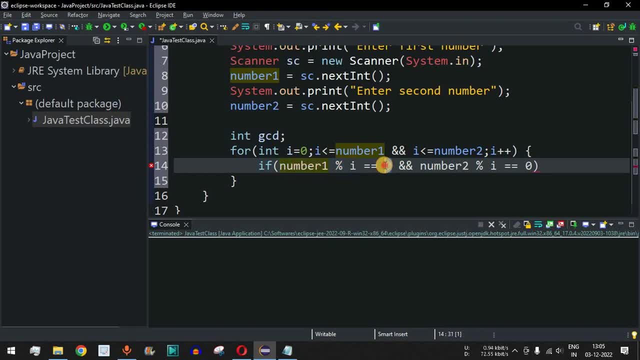 whether this number, that is the first number, percent I, is it giving us the value that is 0, which means a remainder is 0, or not, in which case the number 1 will be perfectly divided by this: I number and number 2 percent I is equal. 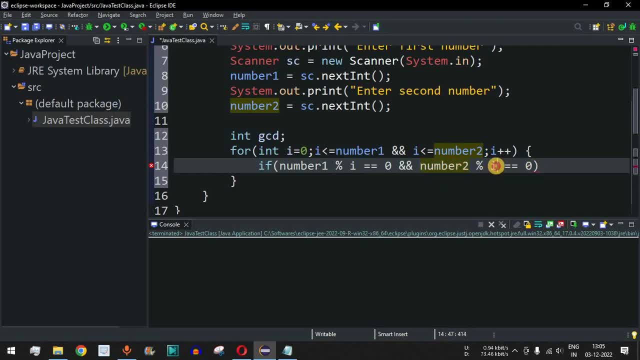 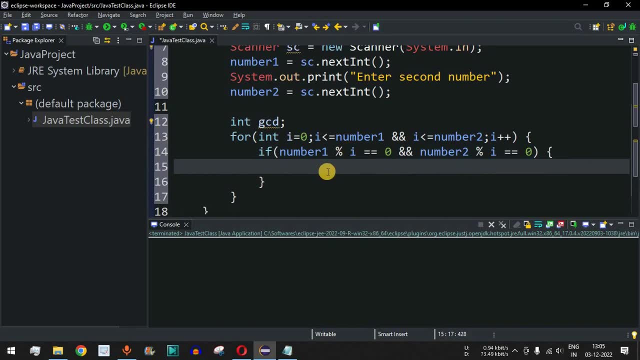 to 0, in which case the number 2 will be also perfectly divided by this number, that is, I. so if this case is true, that is, both these conditions are true- we will say: GCD is equal to this number. that is I over here. so GCD it is equal to I. and then we have semicolon. now, guys, after, 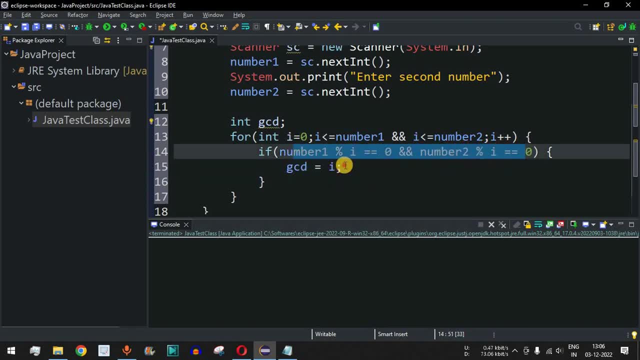 this condition, we also have to check whether the other numbers, that is greater than this particular GCD, whether it is the GCD of both these numbers or not. so again and again the control flow will go back to this for loop and it will go until this condition, that is, I's value, should be less than both the 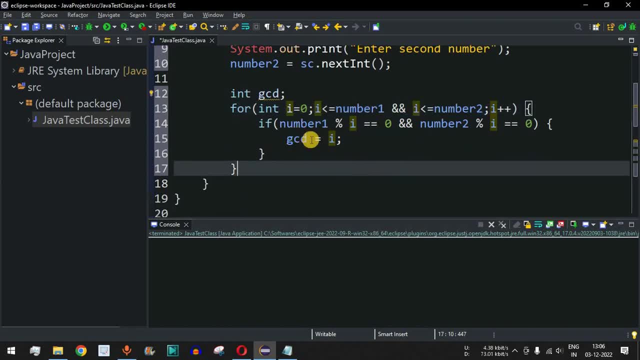 entered numbers over here and ultimately we will find the GCD of both the numbers and what we will do is we will simply print the GCD of the two numbers. so we will say GCD. it is equal to. the number is stored in the GCD variable. 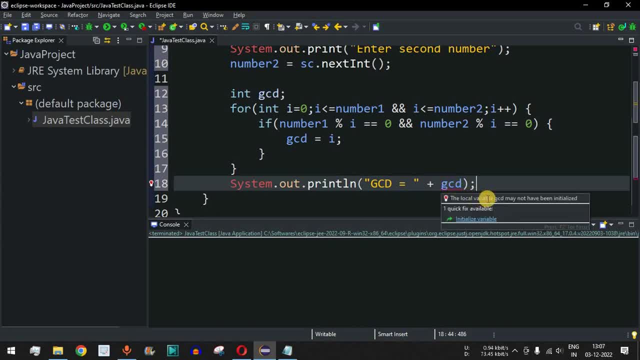 over here. so, as you can see, we are getting a red underline over here. it says the local variable GCD may not have been initialized. so what we can do is simply we can initialize it to one over here. that's because one can divide any number. so, guys, let me just save this file and try running this code now, so as 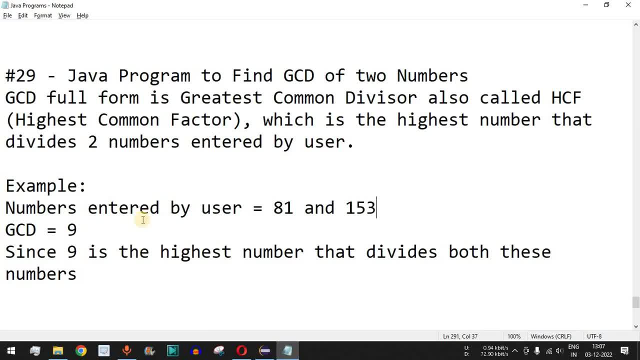 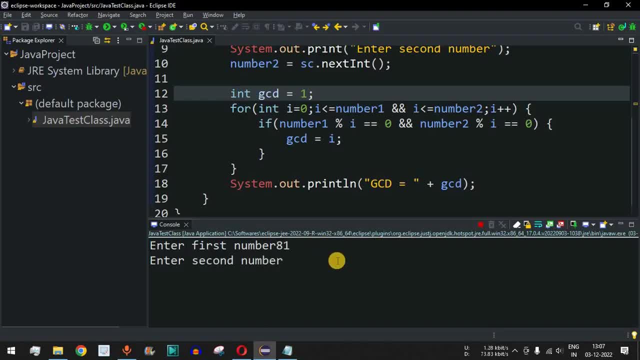 you can see it is asking for enter first number. so what we will do is, let's say we provide these numbers over here, that is, 81 and 153. and the first number we provide it as 81 and then we press Enter. and the second number we provide as 153 over here and when we press Enter it says exception in 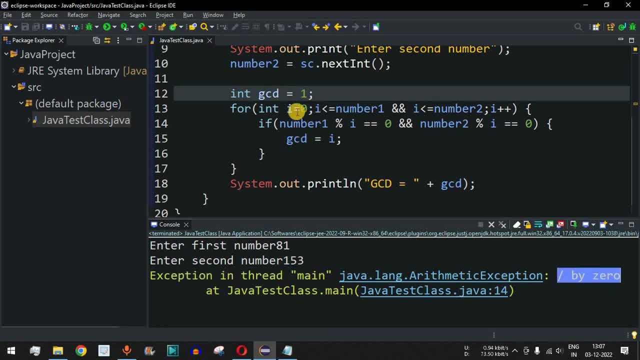 thread main. so divide by 0. so, guys, this is because we have started the I's value as 0 over here, so instead of 0 we will provide it as 1, because any number divided by 0 will give us the arithmetic exception in any Java program. so, guys, 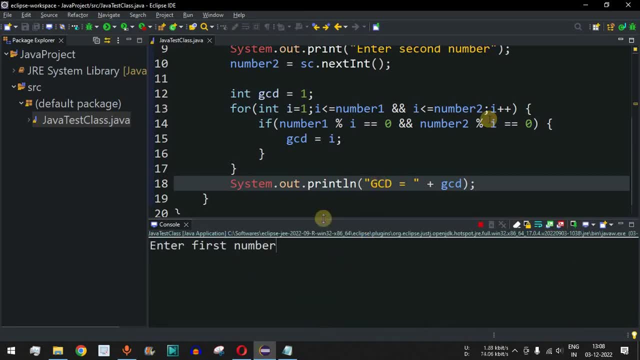 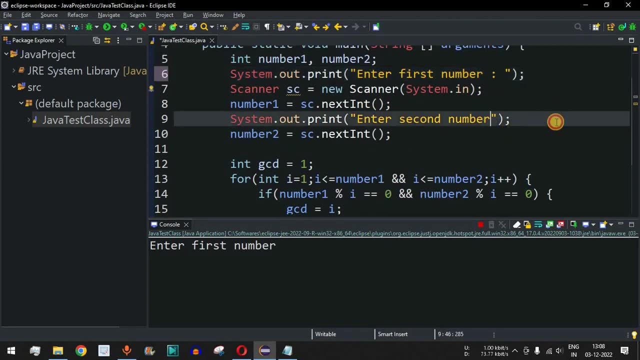 let me just save this file and try running this code now once again. so over here we are getting enter first number, but we are not getting any number over here. so we are getting enter first number, but we are not getting any equal to or colon symbol over here. so i'll simply provide the colon symbols in both. 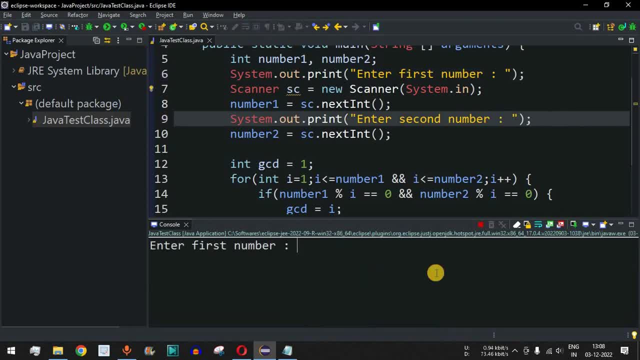 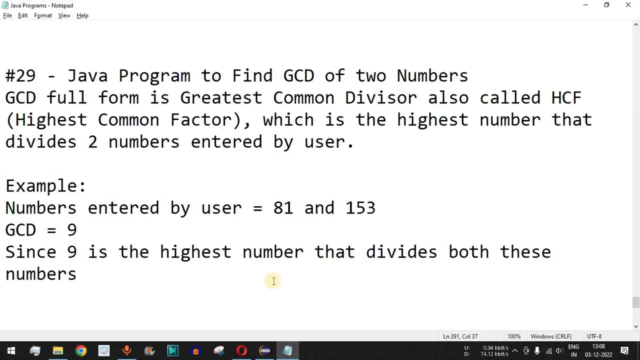 the print statements. let me just save this file and try running this code once again so that it becomes more readable to the user. so we provide 81 and 153. over here we say 81 and the second number it will be 153. i'll press enter as you can see. gcd, it is equal to 9 and that is what we. 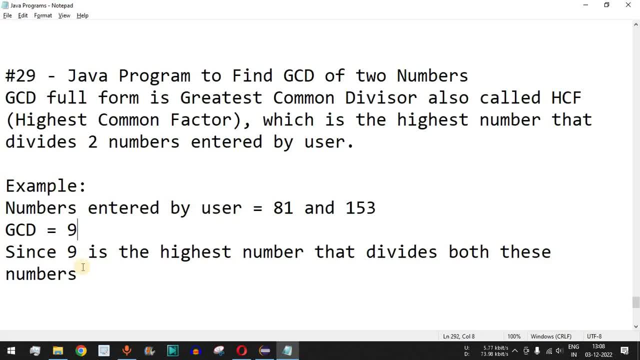 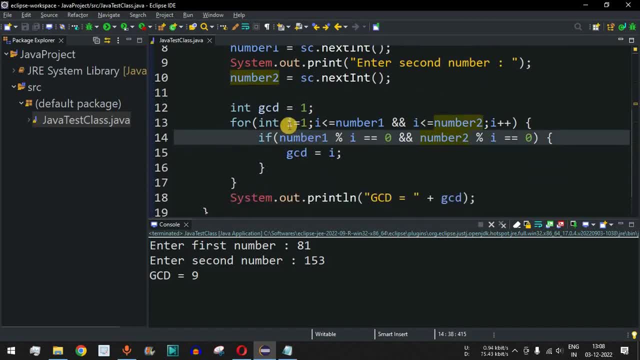 wanted. that is the result. is gcd equal to 9? in this case? that's because it is the highest number that divides both these numbers. now, guys, if you notice over here the for loop, it is going from 1 up to. it is going to 9. so it is going 9 times over here. so it is not one of the optimum codes in. 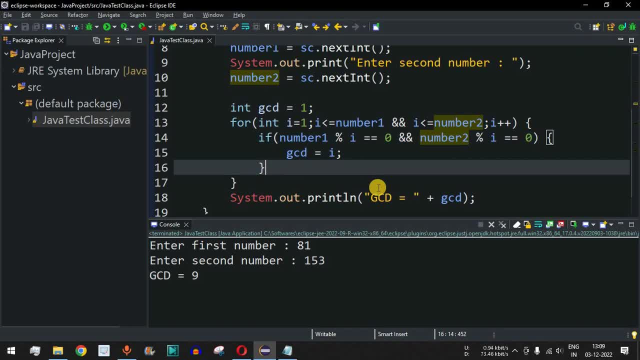 order to find the gcd of the two entered numbers. so one more thing that we can do is another logic in finding the gcd of two numbers is by using the while loop. so in that case what we will do is i'll simply remove these lines of code over here, so we can simply use the while loop. 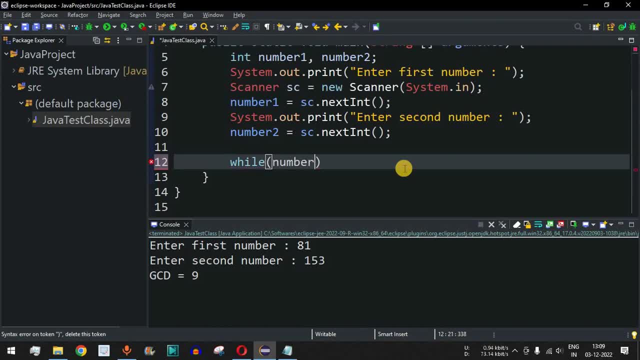 over here so we can simply use the while loop over here. so we can simply use the while loop here and in the while condition we will be having number one. it is not equal to number two. so if any instance, if both these numbers are equal, the control flow. 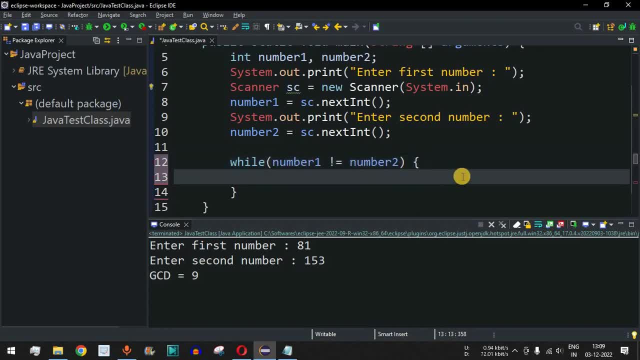 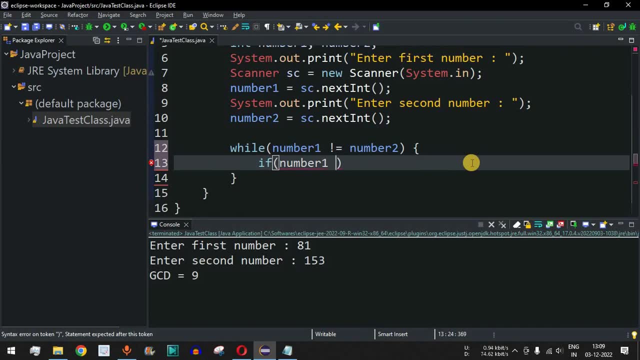 will come out of the while loop. so over here, inside this, what we will do is we will check whether this number one, is it greater than number two over here. so we will say number one greater than number two. so in this case, if number one is greater than number two, so what we will do is we will simply subtract number two. 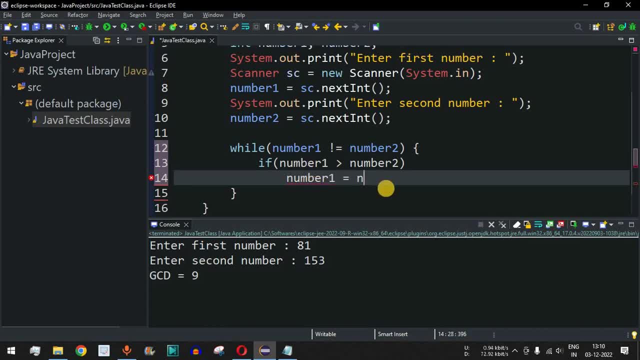 from number one, so it will be number one. it is equal to number one minus number two in this case. so, guys, this is one of the logic behind finding the GCD. in case number one is greater than number two, we will say number one, it is equal to. 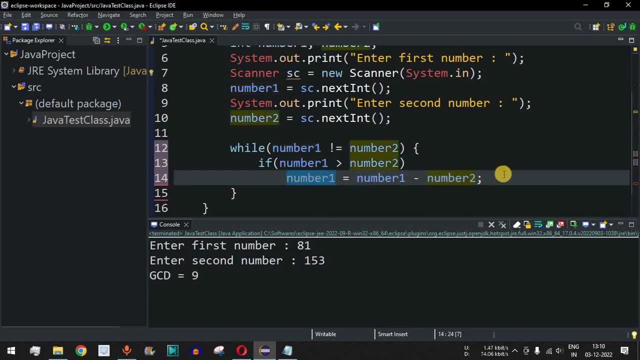 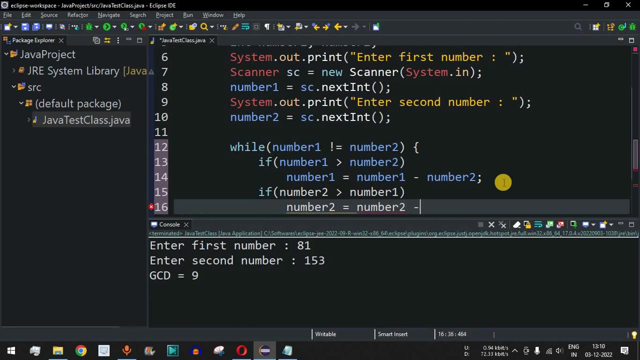 number one minus number two, which means we need to reduce that number. and then in another case, let's say, if number two- over here we say number two is greater than number one in this case. so what we will do is we will say: number two, it is equal to number two minus number one. so we simply need to. 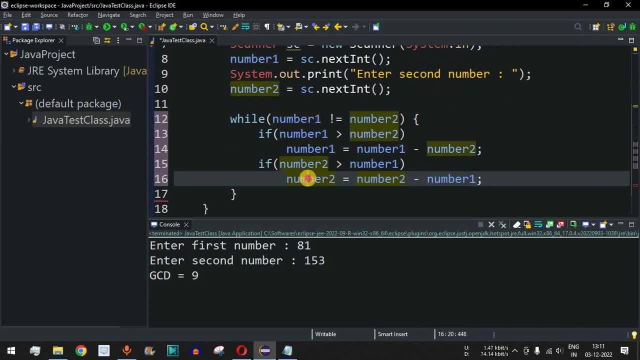 subtract that number one from number two over here and assign it back to number two. so ultimately, guys, we will find a number in such a way that both these numbers, that is, number one and number two, will be equal and that will be our GDC in that case. so once both these numbers are equal, the GCD will be. 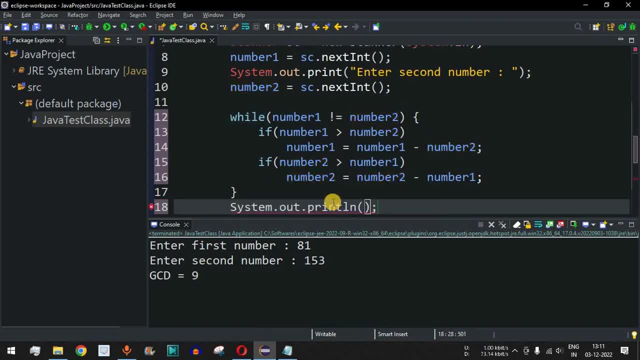 equal to these numbers. so we can simply print one of the numbers in our case over here. so we will say GCD, it is equal to number one. we can also use number two in our case. so, guys, let me just save this file and try running this code now. 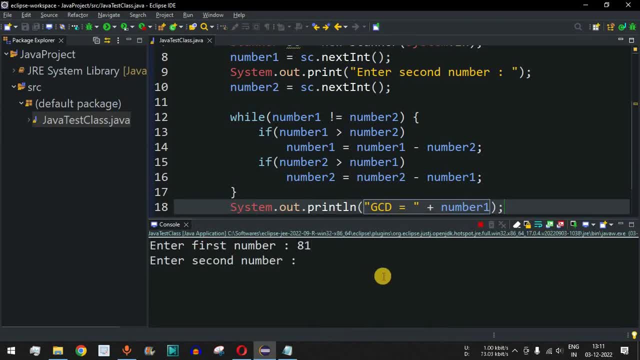 so enter first number. we will say 81. enter second number. let's say we take the same example, that is 153. as you can see, GCD is 9 guys. let us take another example over here. I'll run this code once again. let's see if the number 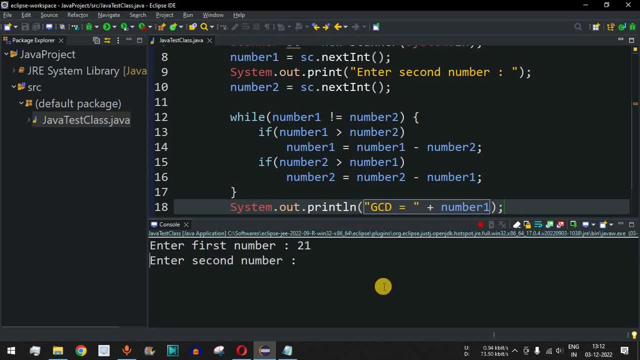 entered by the user is 20.. 21, that is the first number, and second number, let's say, is 49. so probably seven is the highest number that will be able to divide both these numbers, that is, 21 and 49. which is 7 multiplied by 3 is 21. 7 multiplied by 7 is 49. so let me press.